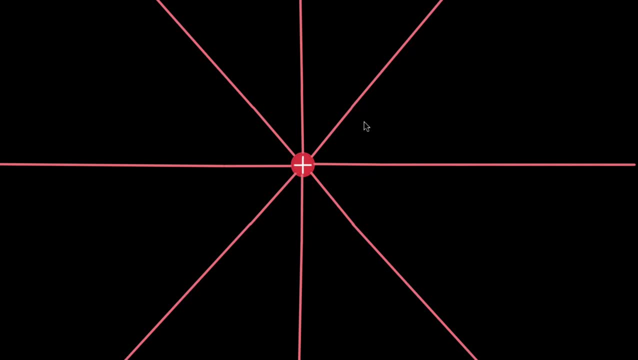 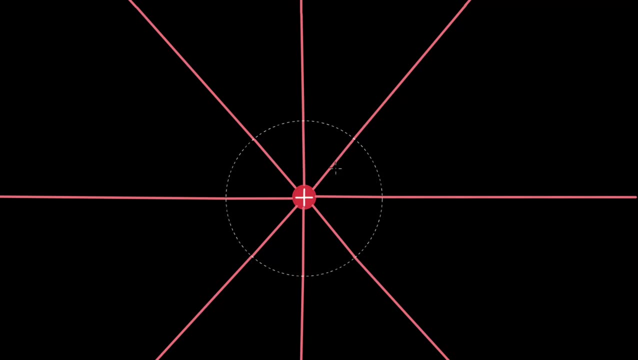 let's say it travels at a speed of 10 m per sec. So that means that the message that the charge has accelerated it must have reached all the points at a distance of 10 m from the charge, And this looks like a positive charge. 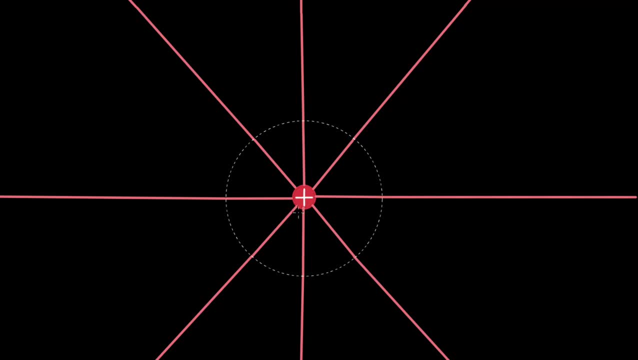 This looks like a circle but it is actually a sphere. So the electric field lines within this region, this sphere, they accelerated with the charge, They remained stuck to it. But the field far away, outside this sphere of 10 meters radius, has no idea that the charge. 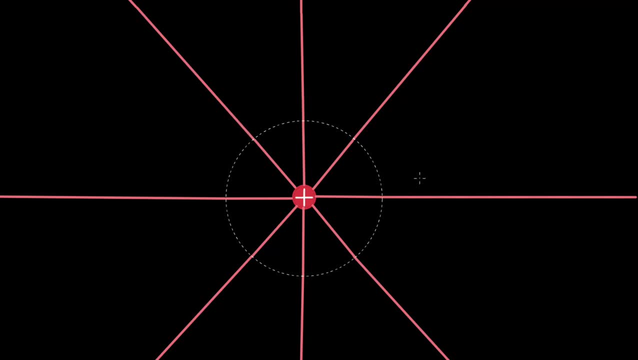 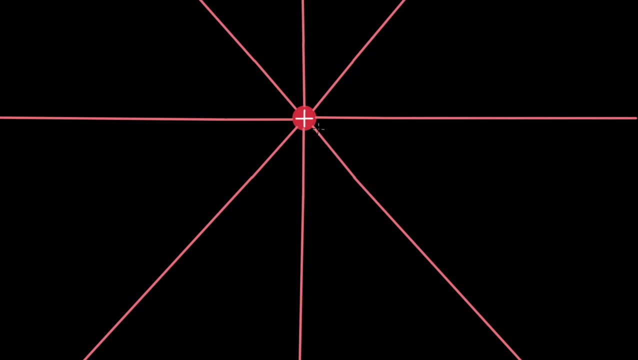 has accelerated. So the electric field outside this sphere is exactly the same when the charge was in its initial or original position. It is still in the old state. Let's see how that would look like. So we start from the original position and we accelerate the charge downwards quickly. 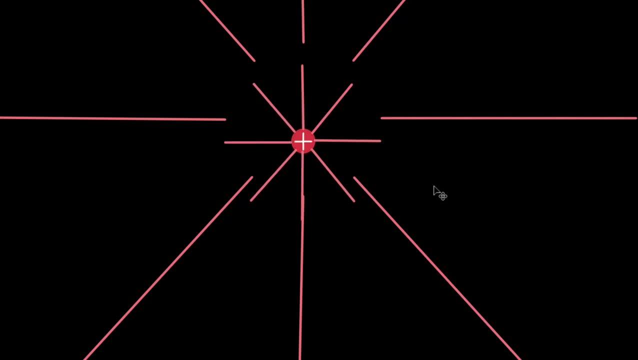 So let's do that. Whoa. So what do we see over here? The field near the charge accelerates with the charge, but the field far away doesn't, because the information of acceleration hasn't even reached them. But these field lines near the charge, they must meet the field lines at the old state. 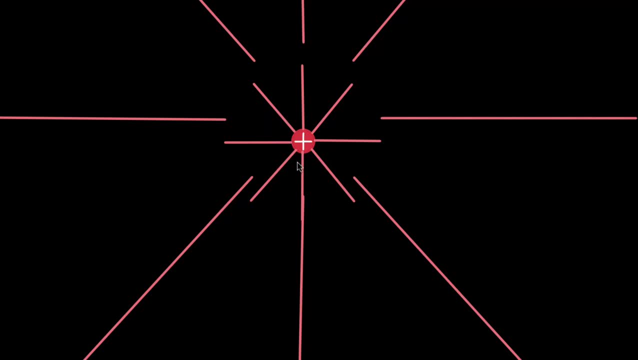 because they are the same field lines, after all. The electric field lines cannot break. So the field between these distances, between these distances they must join. This leads to the formation of kinks. They look like this: There is a kink form here, here and here, but none is formed along the axis of movement. 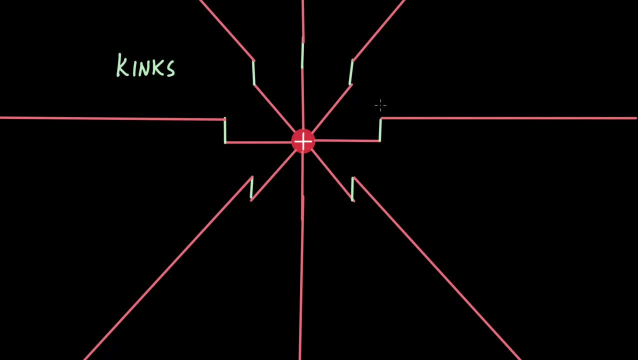 None is formed vertically. It is this kink or collection line. This kink is responsible for electromagnetic radiation that we will see in a while, And these kinks, they move outward with the speed of light. So let's see how that would look like with the help of an animation. 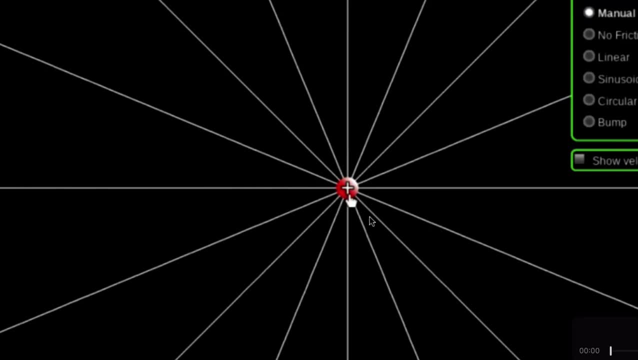 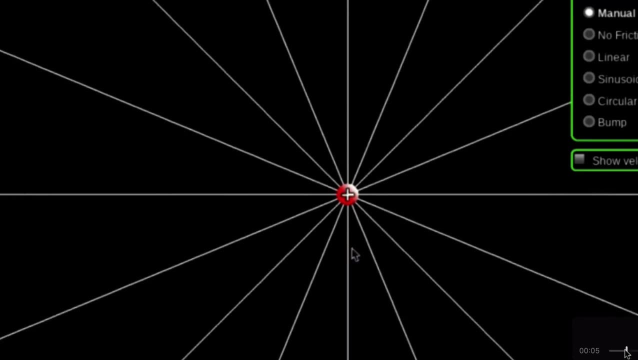 So here we have the same positive charge and this will be accelerated downwards quickly. So when we do that, notice how these kinks move outwards. Let's look at this again. And there you go. All right now, accelerating charges, they produce kinks and these kinks, they move outwards. 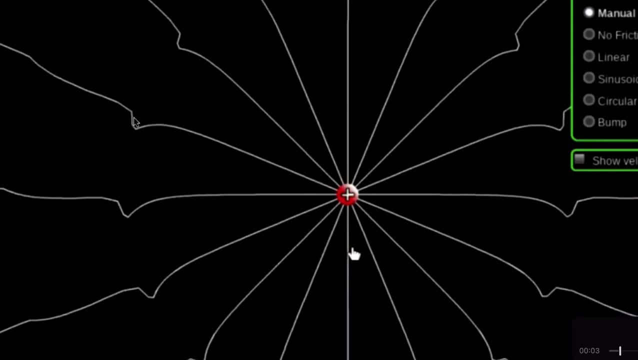 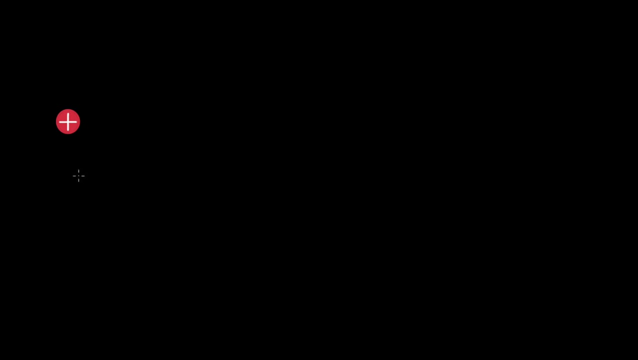 with the speed of light. Now, in order to understand how these kinks might be responsible for electromagnetic radiation, we need to look closely at this region of electric field. Here we have the same charge accelerating downwards, So when it is further down it has some acceleration and also some velocity due to that acceleration. 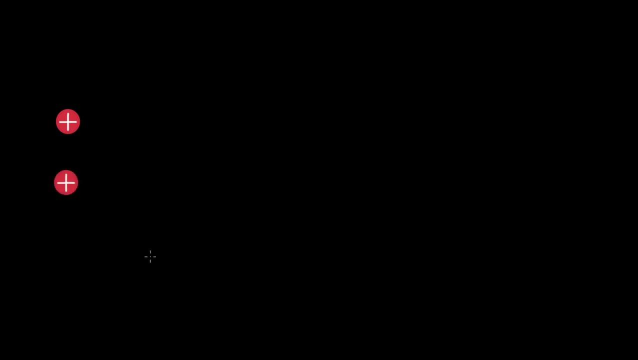 Now let's see where the charge moves. Let's see The charge will be after some acceleration. So let's say: there it is. Now let me draw some field lines, and in this case I'll draw only one. So for the charge at its initial position, let's say that the field lines one field. 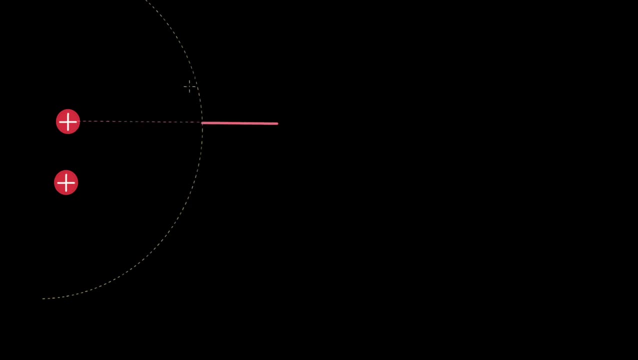 line goes radially outwards like this. Now, the region of space outside this sphere has not received the information that the charge has accelerated, So it stays where it is, whereas the world inside this circle has changed, And so are the electric field lines with it. 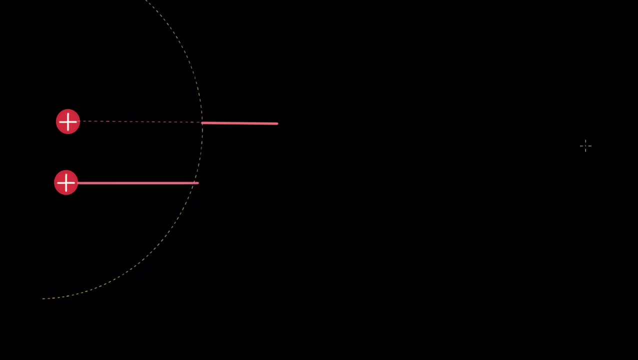 Okay, So the electric field line inside the circle, it goes along with the charge and it looks like this: And this will result in the formation of a kink because the electric field line has to join. So the kink looks like this. 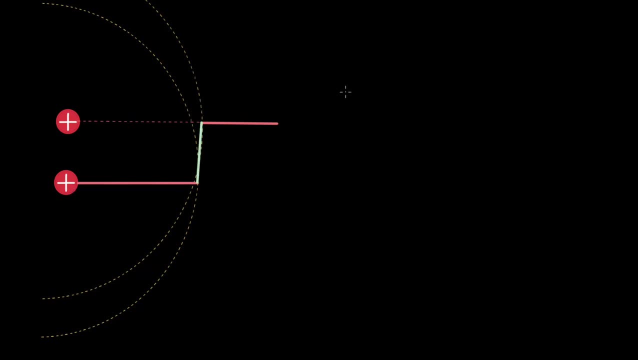 And now this is the electric field line. This is how it goes. Now we can see that this electric field line in the region of the kink is. it is at some angle And we can actually resolve this into components, So it will have a perpendicular component. 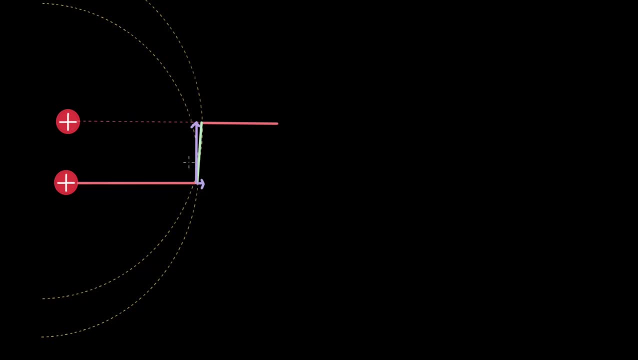 And it will have a radial component. Okay, So this is the perpendicular component of electric field. It is this perpendicular component of electric field in the traveling wave that is part of the electromagnetic wave that moves outward with the speed of light. If you're looking at the wave from here and this whole shell comes over to us, it is only 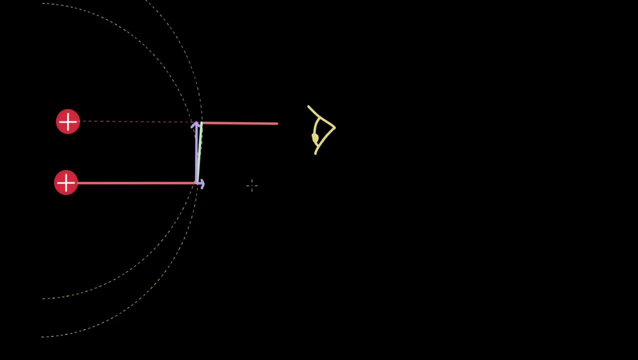 this perpendicular electric field in our line of sight, which we can see as moving outwards. Now, what could the magnitude of this perpendicular electric field depend upon? We accelerated the charge, And that produced a kink in the electric field And, upon resolving it into two components, we obtained the perpendicular component and 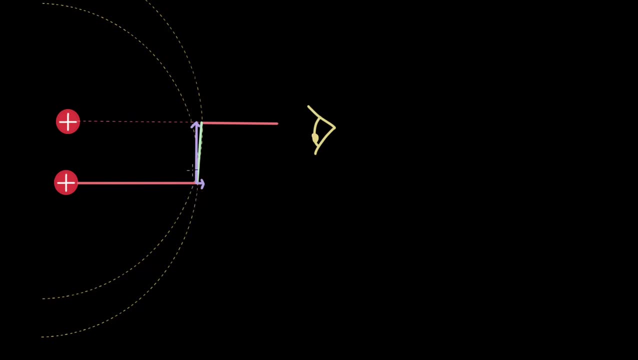 a radial component. Maybe if the kink is even bigger in size, then the perpendicular component might even be longer. What could lead to a bigger kink? Maybe let's try and provide some more acceleration to the charge and see what happens. So let me remove the charge at this position. 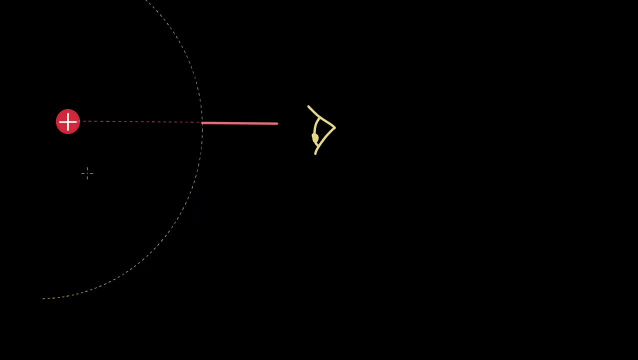 So let's start from the initial position and provide greater acceleration to the charge. So the charge might be somewhere over here. now It has moved further down because it has a greater acceleration. In this case, the electric field that goes along with the charge can look like this: 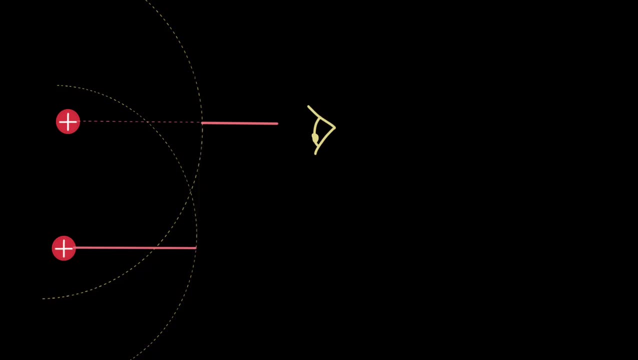 Now, if we, if we join these electric field lines, we will see that the kink formed in this case is slightly longer, is slightly bigger And upon resolving this kink into components- the electric field and the kink into components- this is how the components could look like. 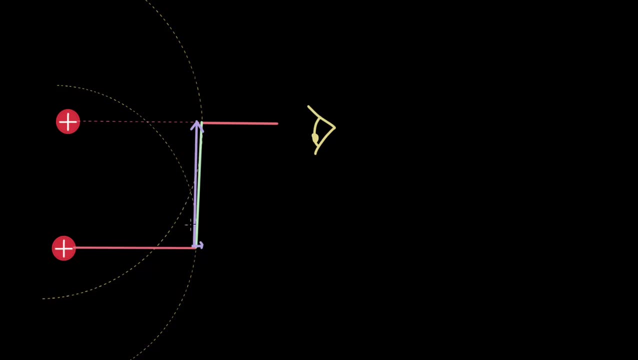 And we can see that the perpendicular component, the magnitude of the vertical component, is bigger in this case, And that happened when we provided the charge with greater acceleration. So if the charge accelerates with a greater magnitude, we get a bigger electric field. 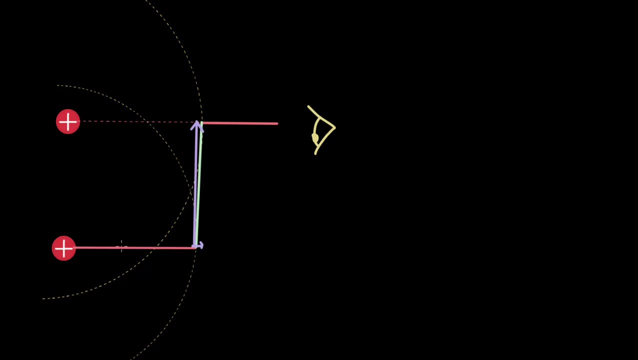 which propagates again outwards with the speed of light. Now, so far we have been accelerating the charge downwards. Let's accelerate it upwards and see what happens. So now we are starting over here at rest, And then we will accelerate the charge upwards. 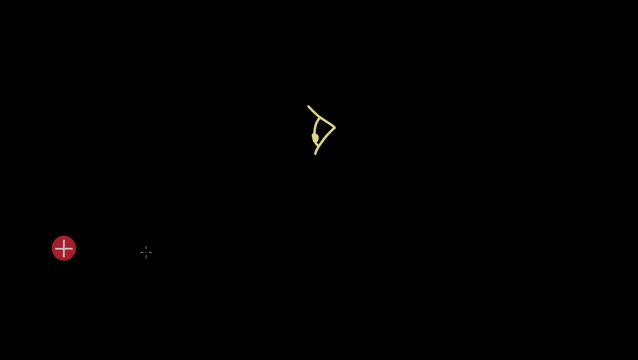 Let's see what happens At this point. the electric field lines- and I'll draw only one- will look like this, And then, when we accelerate it upwards, maybe the charge is over here now. So when the charge is over here, the electric field line inside the circle will move along. 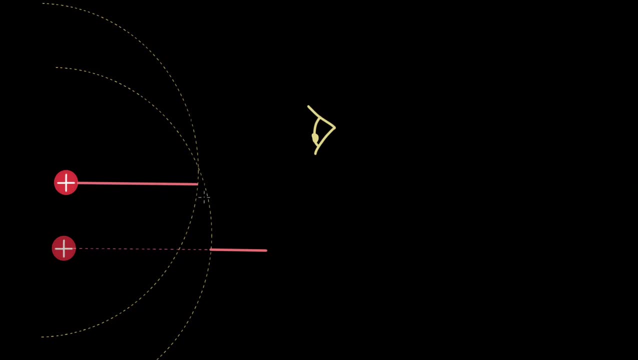 with the charge. So that could. that could look somewhat like this, But again we can see that there will be a kink formed now because the information of acceleration outside the circle has not reached the electric field. They don't even know. 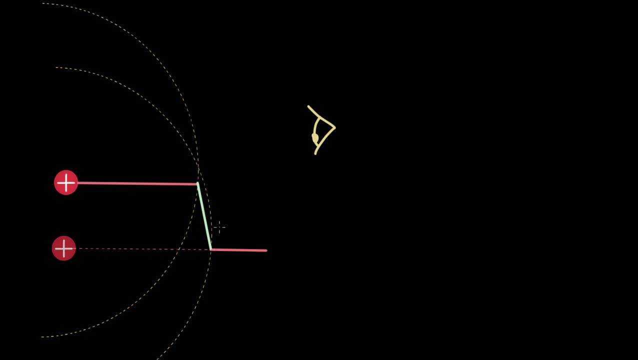 So, as a result of which, A kink is formed in this direction, And now the electric field goes like this: from this positive charge go down and then go out. So if we resolve the electric field in this kink region into components, this is how the 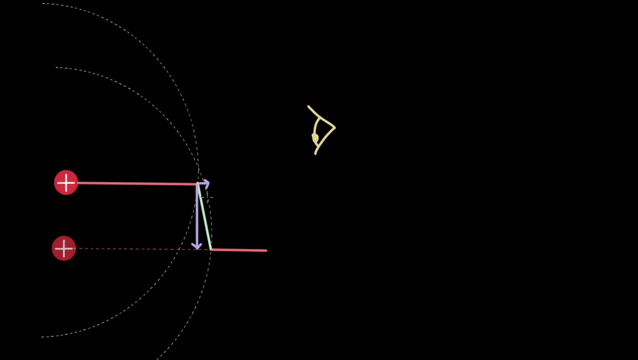 components will look like. Here we see that the perpendicular component of the electric field is pointing vertically downwards. So when we change the direction of acceleration, even the direction of the vertical component of the electric field, the perpendicular component that propagates outwards, even that direction, 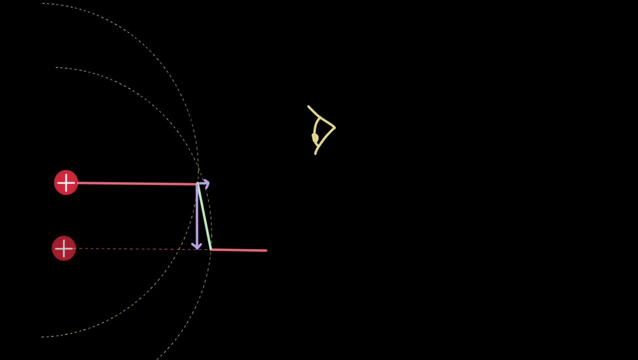 changes. And if we were to oscillate the charge sinusoidally? that is, changing the acceleration of the charge sinusoidally, which means it increases, then it becomes zero, then it decreases and increases in the opposite direction. the magnitude of the electric field should change according. 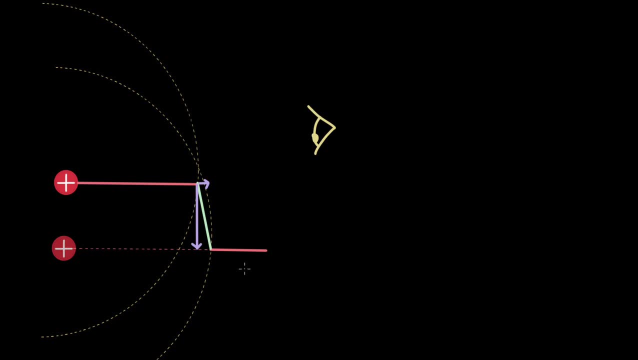 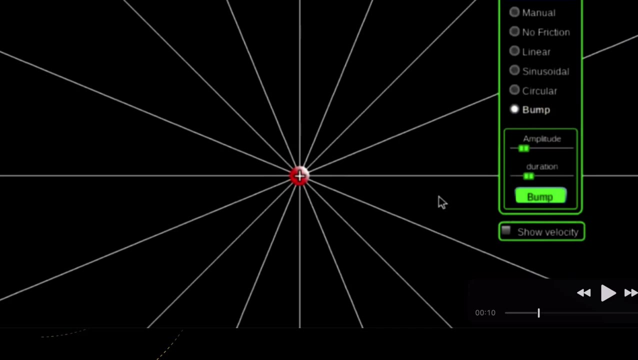 to that as well, And it should change its direction when the direction of acceleration changes. Let's take a look at all of this in an animation Now. if we provide a bump that is accelerating downwards and then quickly upwards, the direction of the electric field vector must change. 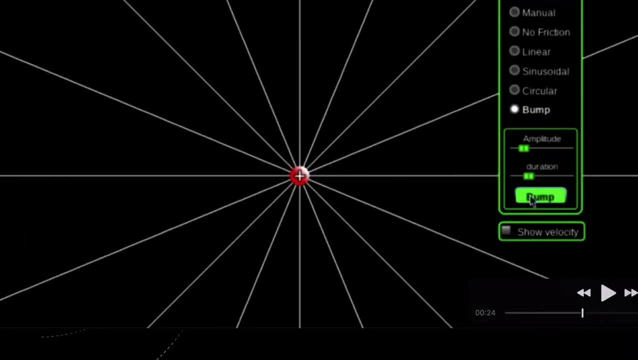 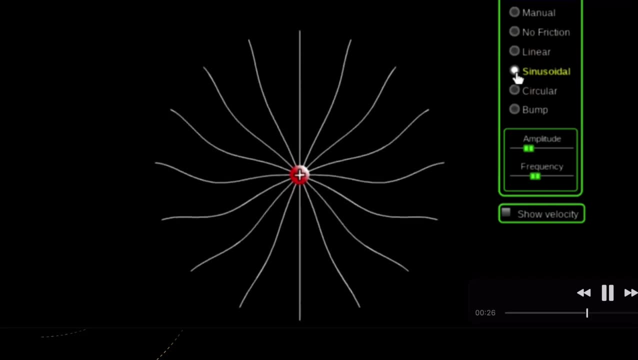 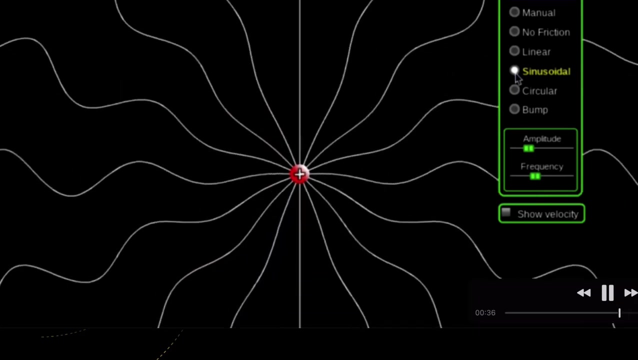 So let's see how that will look like. There you go Now. if we oscillate the charge sinusoidally, we should see kinks that look like sine waves. If we increase the frequency, that is, if we oscillate it faster, we see the sine waves. 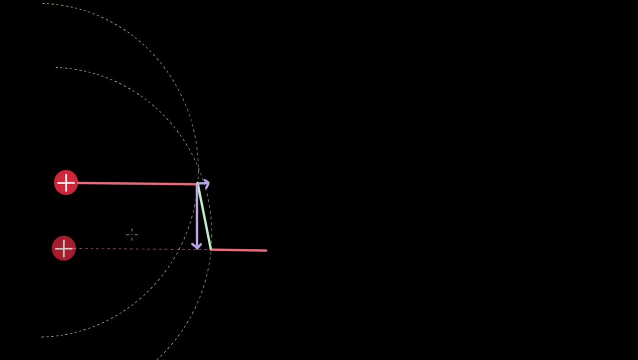 clearer in this case. All right, now, where does magnetic field come into picture? We can say that the charge is moving upwards. If the charge is moving up, so there can be a magnetic field due to that movement, because we know that moving charges produce magnetic fields. 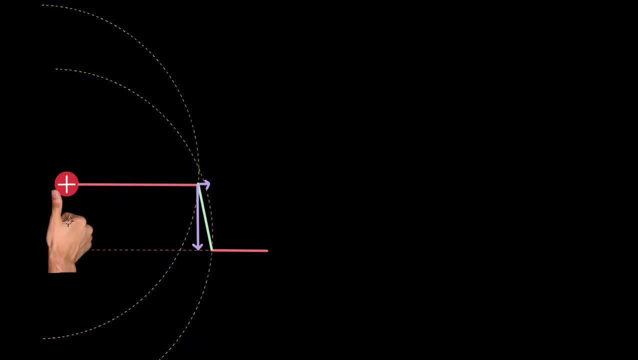 And if the charge is moving up, using the right hand rule, pointing a thumb in the direction of the movement of the charge can give us the direction of the magnetic field, and that is given by the curl of the fingers. But it turns out that the magnetic field that is produced due to the movement stays alive. only for very short distances, But for distances Far away From the source. The magnetic field that is induced is due to the changing electric field, And it is the electromagnetic radiation, far off from the source that is useful to us, that is even detected. 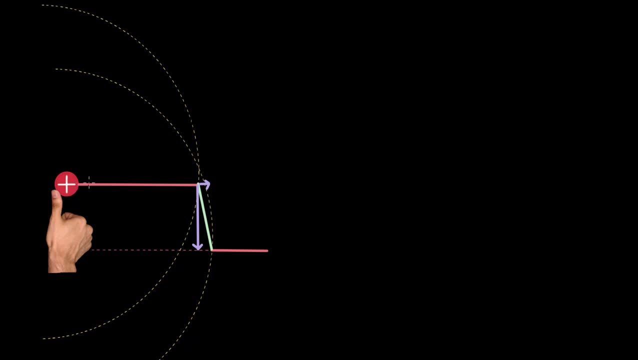 The magnetic field that is generated due to the movement dies very quickly close to the charge. So if this electric field vector is moving to the right, it will create a magnetic field that is perpendicular to it And we can figure out the direction of magnetic field. 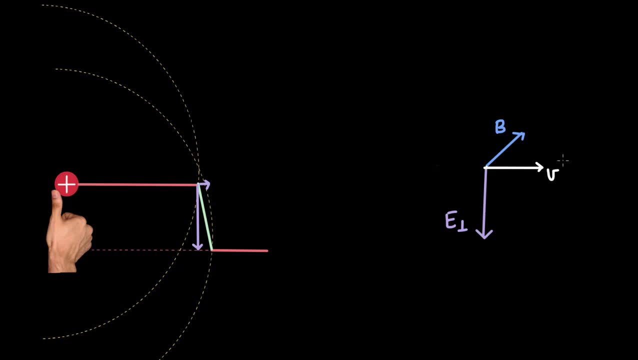 So if this electric field vector is moving to the right, it will create a magnetic field or electric field or even velocity. If we know 2 out of these 3 vectors, The direction of the wave travel is always in the direction of E x B. 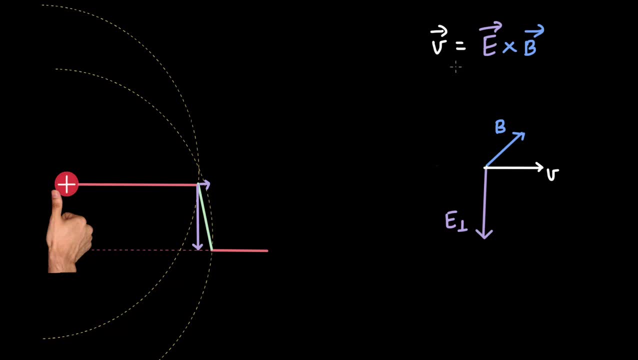 This is the direction of the wave travel or the direction of velocity. So in this case we knew that the wave was moving to the right And the perpendicular component of the electric field is vertically down, So the magnetic field vector had to point away from us, into the verbose места. 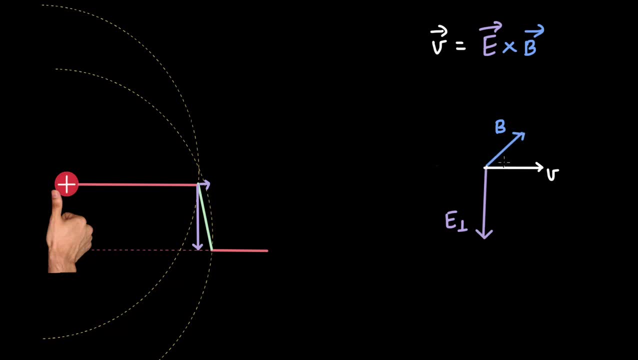 The magnetic field vector was moving to the right. The magnetic field vector is pointing into the direction of the wave travel. It was moving to the opposite direction, the plane of the screen. because if we take the cross product, if we take the cross product and 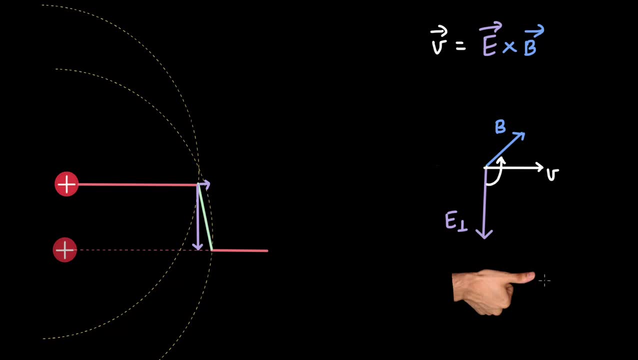 use the right hand rule. in this case, the thumb would be pointing to the right and the curl of the fingers goes from the electric field to the magnetic field when the electric field vector was pointing up. even then, the wave was moving to the right and in that case the magnetic field would 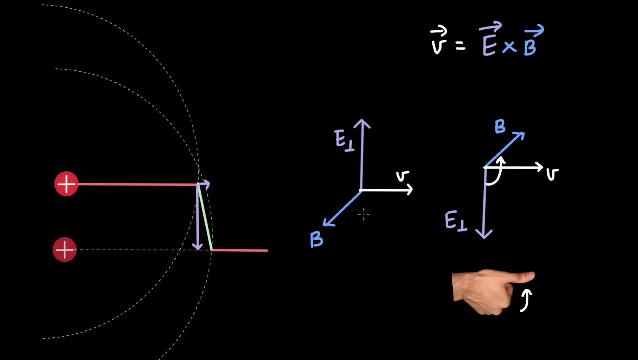 be pointing outwards, and we can use the same right hand rule to confirm that. so our thumb should be pointing in the direction of the movement of wave. and again our fingers. they go clockwise, they go from e to b, e cross b, and the direction of e cross b is the direction of wave travel, so far off from 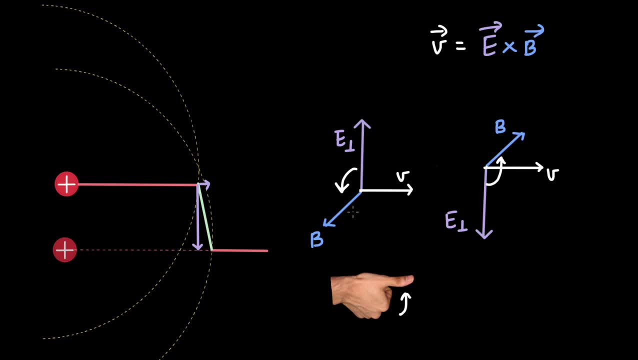 the source, it is induced electric field that induces a perpendicular component of magnetic field. let's see how this looks like in three dimensions. so here we have the charge, and in this case we are again only accelerating the charge in the downward direction. we are not accelerating the charge in the downward direction, we are not accelerating the charge in the downward. 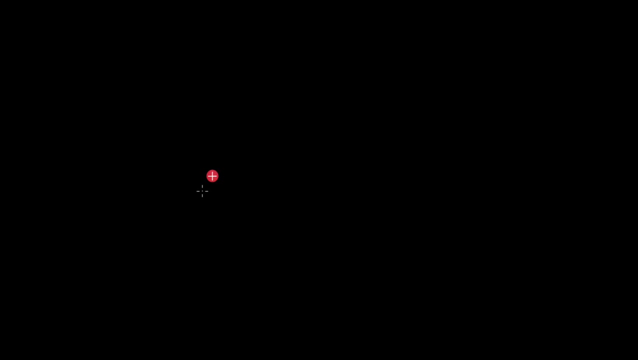 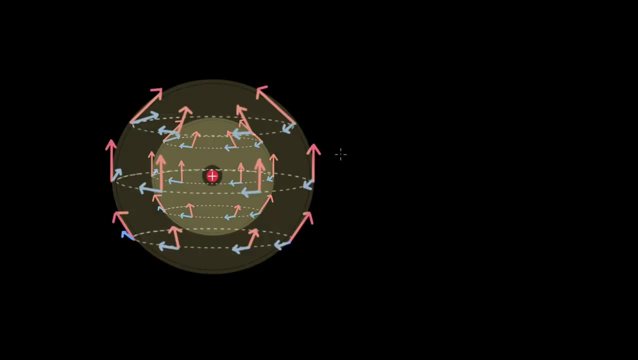 direction. we are not accelerating the charge in the downward direction, we are only moving it, accelerating it downwards. we see these electric and magnetic field lines propagate in all the directions at the speed of light. so after after some time, these electric and magnetic field lines might have reached this position. they are propagating outwards. and after some more time, 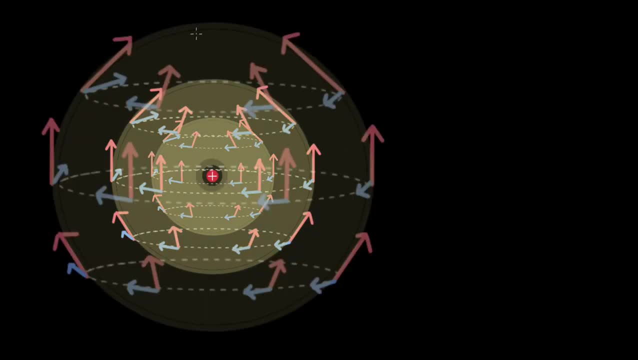 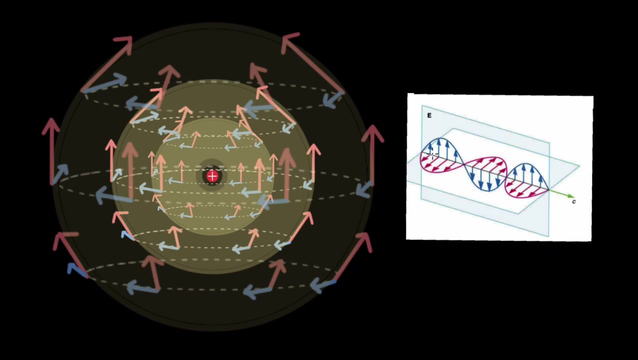 these same lines must have reached at this position. notice: there is no electromagnetic radiation vertically, and we can connect this to what we saw earlier, because there is no kink formed in this region, so there is no electromagnetic radiation over here now. usually in textbooks we see an image somewhat like this: a sinusoidal nature of electromagnetic waves. this is 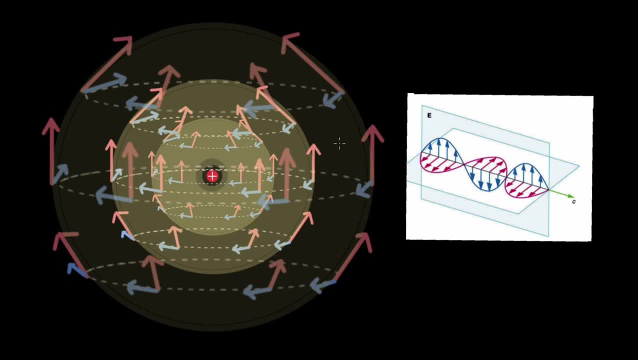 what we get when we oscillate the charge sinusoidally, that is, when the charge is accelerated downwards, we will see electric field vectors which are pointing in the upward direction. and as the acceleration changes, so does the magnitude of the electric field vectors. and when the acceleration changes its direction, so does the direction of the electric field vectors. 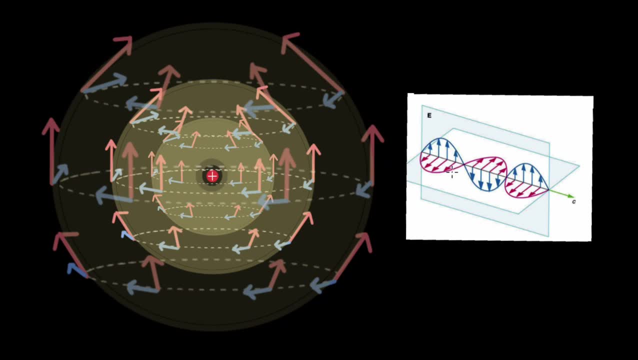 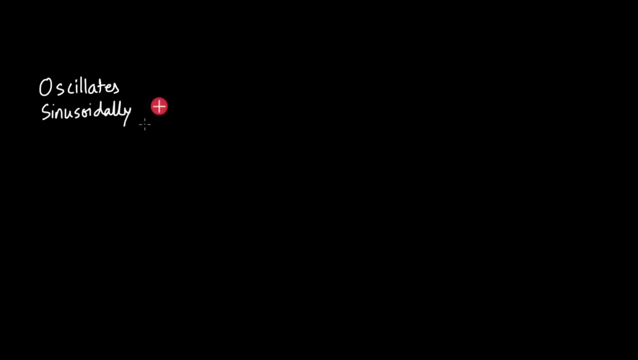 and also the direction of magnetic field changes as the direction of movement of the charge changes. but let's try and arrive at this image that you see on the right. so for that we will have one charge which will oscillate sinusoidally, that is, the acceleration will increase and it will 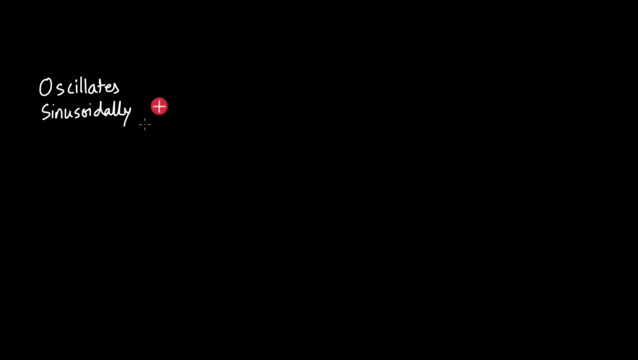 decrease, then it will again start increasing, but in the opposite direction, just like a sine wave. and let's say that the charge is placed at this position and it is oscillating sinusoidally along the vertical axis. now, when the charge has an acceleration vertically downwards, a maximum acceleration downwards, we will 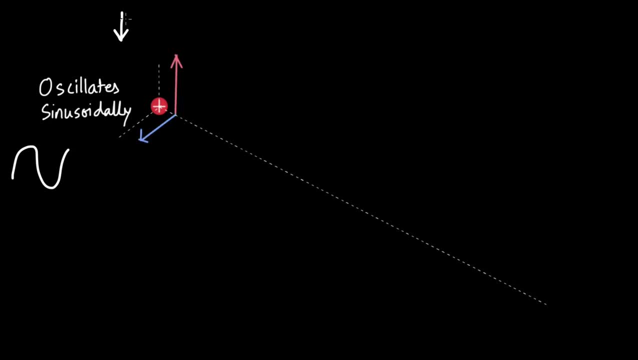 get an electric and magnetic field line somewhat like this: now, when the acceleration changes, let's say if it decreases but it is still vertically down, this electric and magnetic field vector will keep on propagating, it will move forward, but you will have a new electric and magnetic 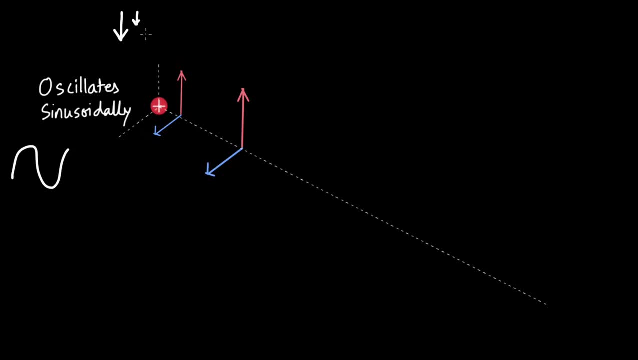 field vector which is smaller in length because the magnitude of acceleration has decreased. let's say, if the acceleration decreased further, so we will have a new electric and magnetic field vector. it is even smaller. now. you will get a smaller perpendicular electric and magnetic field vector and when the acceleration changes its direction, when it when it is in the opposite direction, 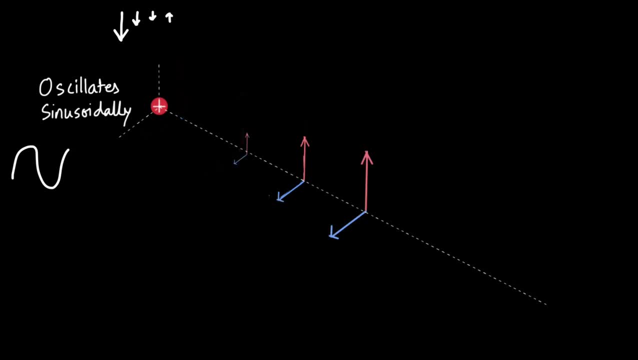 these vectors. they will keep on moving forward with the speed of light. so this is where they are now, and now you have an electric field in the opposite direction because the direction of acceleration changed. now, when the magnitude of acceleration increases further in the opposite direction, you will get a pair of electric and magnetic field vector again, but from the opposite direction. 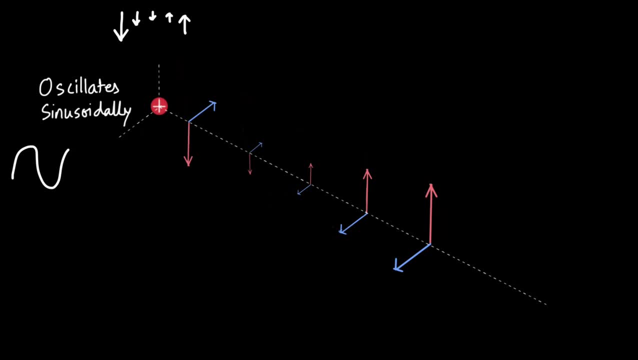 with greater magnitude in the direction shown. and lastly, if we keep on doing this, you will reach a maximum electric and magnetic field vector, just like this. now let's try and join the tips of the electric field vectors and the magnetic field vectors. so when we do that, when we do that for 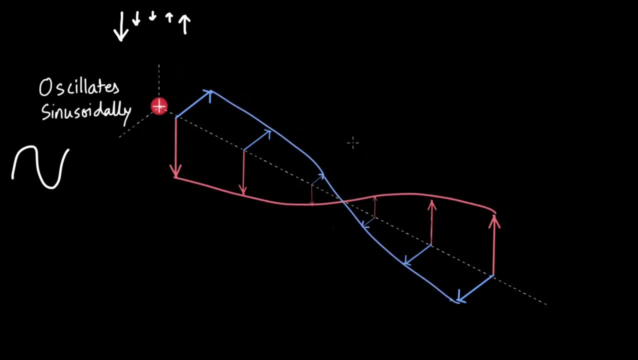 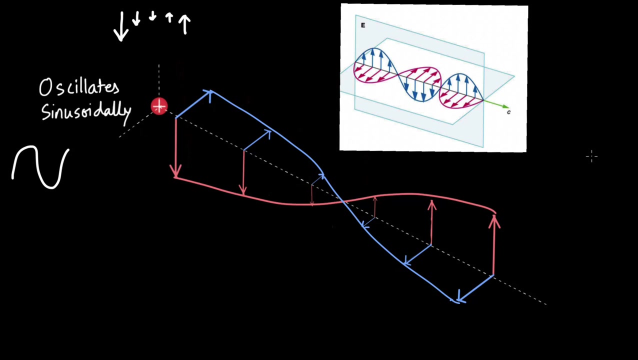 electric field this is how it can look like, and for magnetic field it looks like this: they are perpendicular to each other, even though this is not the full sine curve in the true sense, but you can imagine if it continues it will form a sine curve, just like this. all right, so in this video we 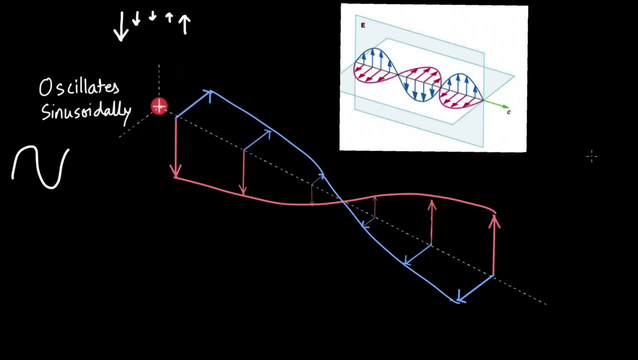 saw how accelerating charges produce electromagnetic waves that propagate or move in all the directions with the speed of light. as a result of the charge's acceleration, a kink is formed and in that region of kink the perpendicular component of electric field moves outward. and it is that changing.